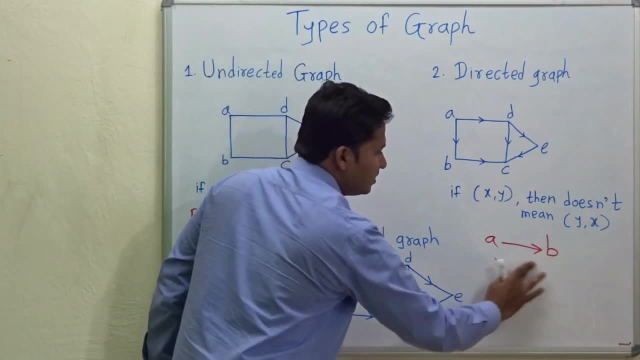 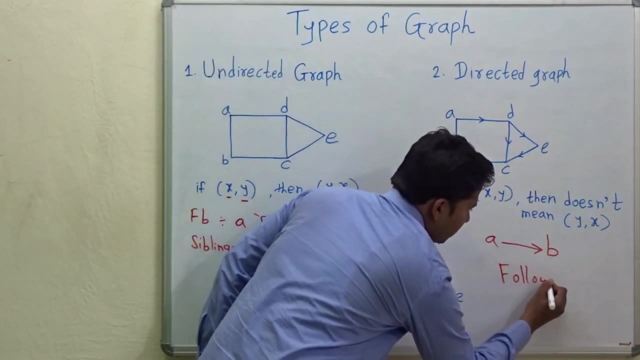 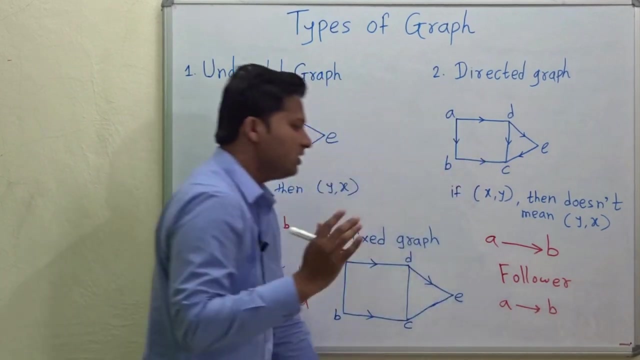 then only there is an edge from b to a. But if it is not, then the edge is not present. So this relationship is like follower relationship on Twitter. Okay, So if a follows b, then it does not mean that b should also follow a. Okay, So this relationship is. 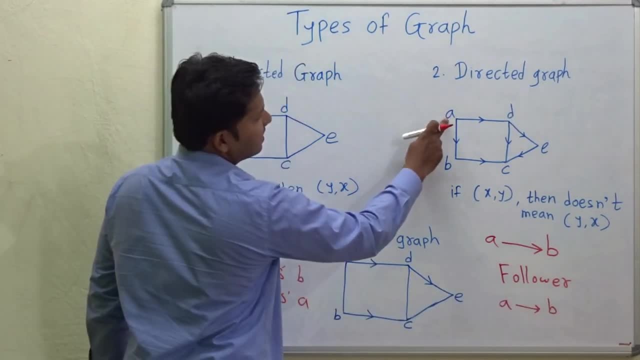 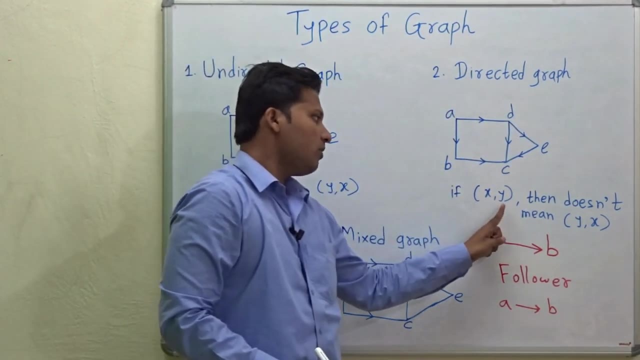 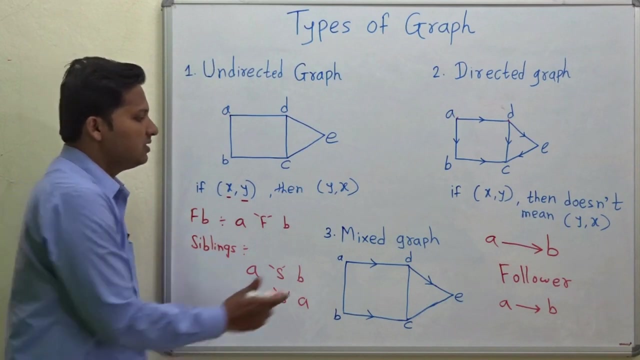 one directional right. So see here, a is connected to d, but that does not mean that there is an edge from d to a. So if x y, then it doesn't mean that y x right. And the third graph type is the mixed graph, So in: 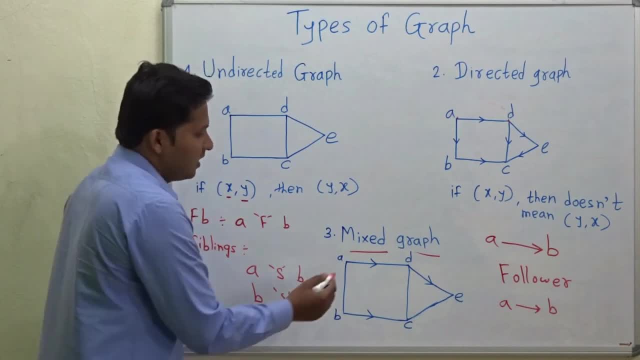 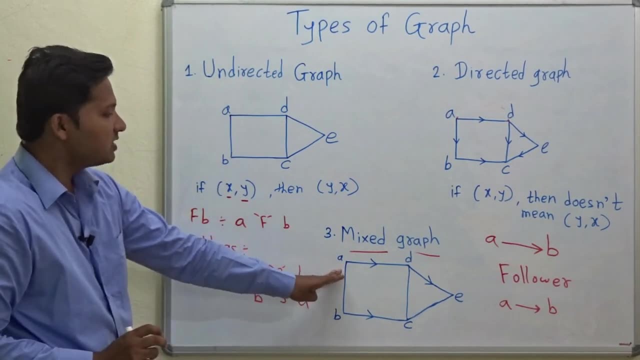 the mixed graph, both edges are present means there is a directed edge as well as there is an undirected edge, right. So the application of the mixed graph is the scheduling problem. So the job scheduling problem. Okay, So the job scheduling problem. 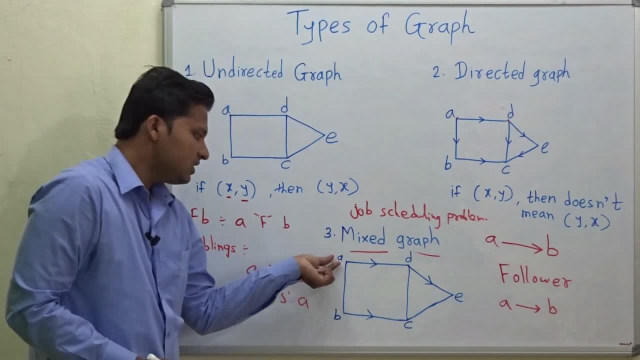 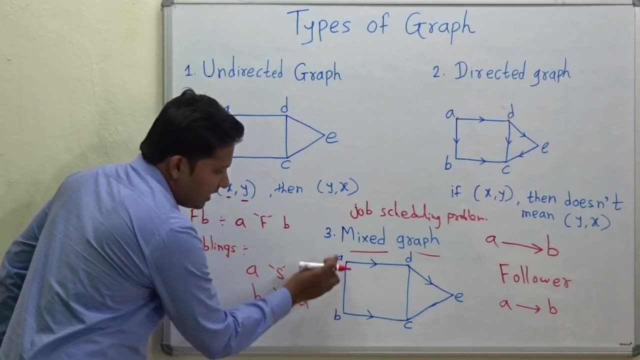 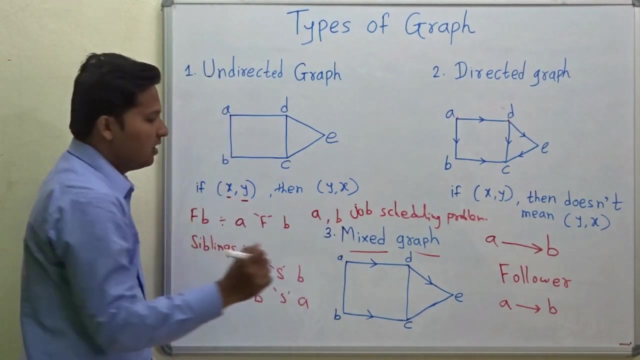 Okay In job scheduling problem. so suppose these are the jobs a, b, d, c and e. Then, as there is no direction from a to b, that means jobs a and b are independent, means there is no time constraint. 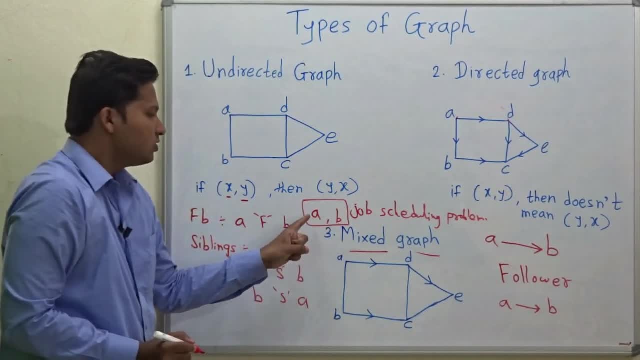 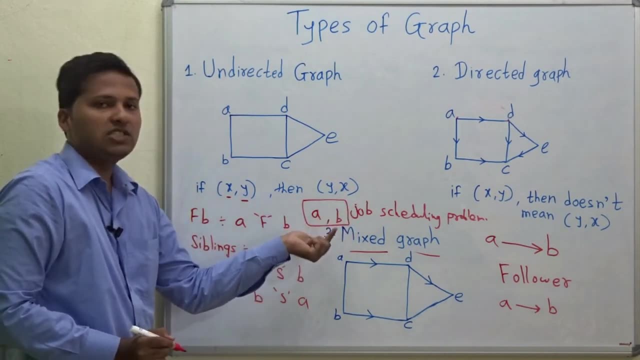 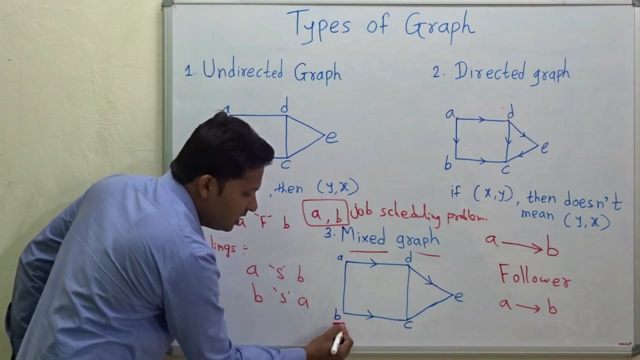 for jobs a and b right. So job a can be done at any time and b can be done at any time means they are not dependent on each other, But there is a direction from b to c. that means only after b is completed, then only job c can be. 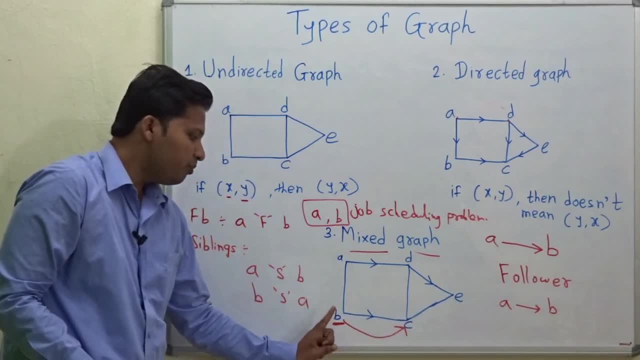 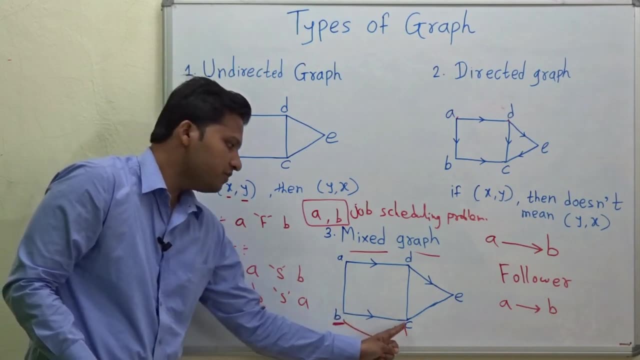 done Right, Because the output of job b is the input of job c. for example, output of job b is the input of job c. So when b is completed, then only job c can be done. This direction tells us that. So say: if a and b 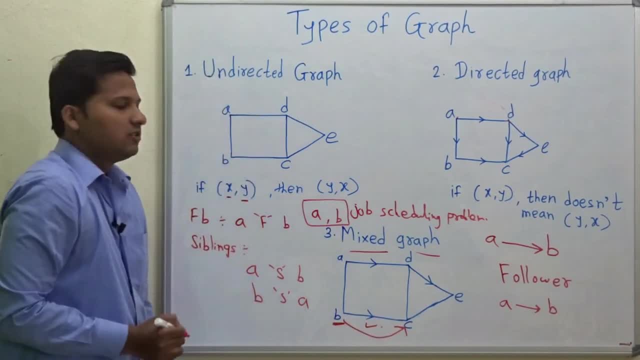 are independent. Okay, So when b is completed, then only job c can be done. This direction tells us that, then only job c. That way only b can be done. This direction tells us that. So two Bodyментity creates Mask. marching Bye, Welcome ego. okay, So so when 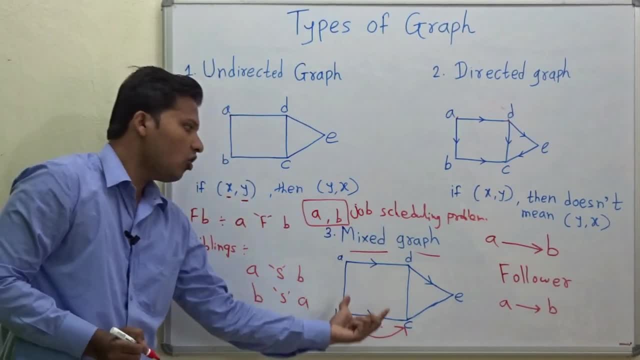 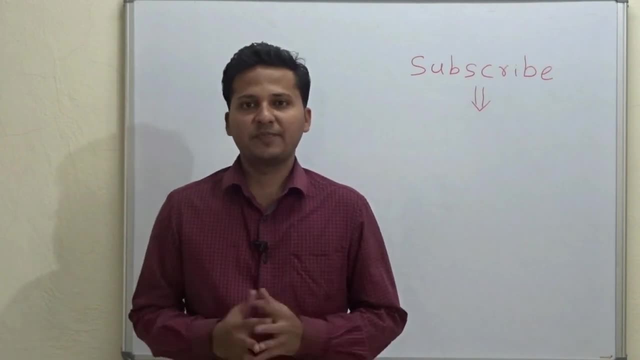 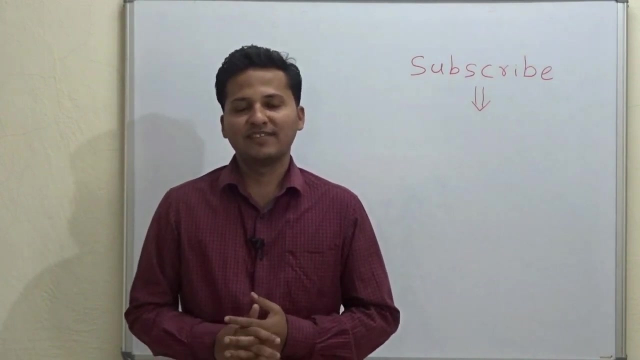 So the scheduling job problem is an example of mixed graph.